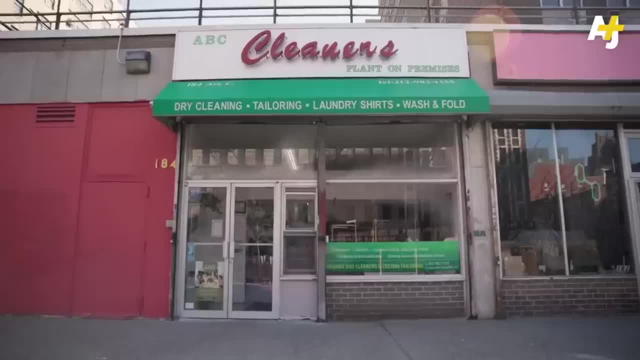 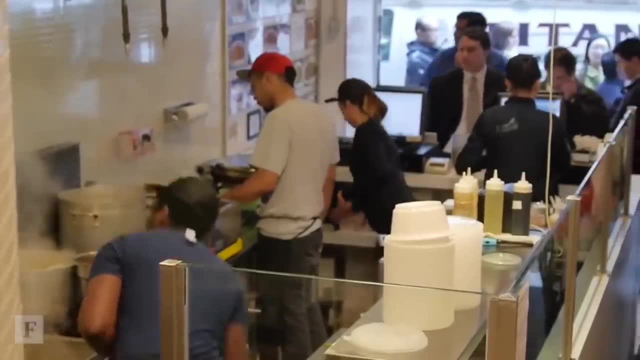 medicine to technology. According to the Asian American Chamber of Commerce of Maryland, Asian American businesses bring in more than half of the revenues generated by all minority businesses throughout the state. Earlier this year, Indian American, a woman named Aruna Miller, became Maryland's 10th Lieutenant Governor. becoming the first Asian American to hold a statewide position. Number 9 is Massachusetts, with 7.7%. The dominant ethnic group is Chinese and live mostly in Boston and its suburbs. From 2000 to 2010,, a Boston suburb, Quincy, had its Chinese population increase by almost 60%. 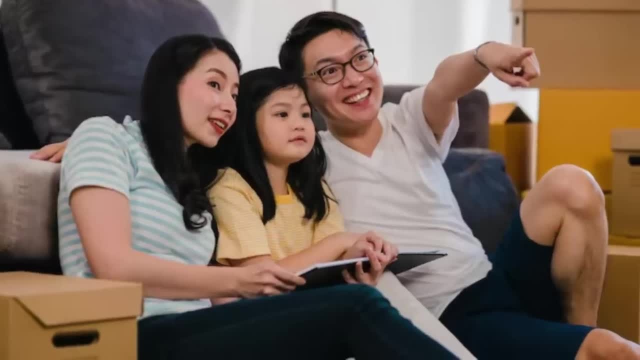 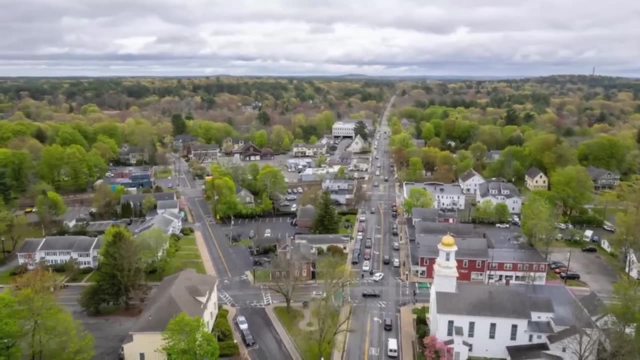 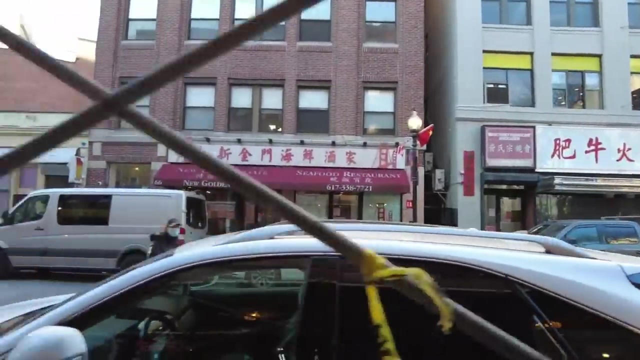 As of 2000,. 65% of the Chinese in Quincy were homeowners. Acton, a suburb just north of Boston, had a 151% increase in Chinese immigrants from 2000 to 2010.. Downtown Boston's Chinatown is the cultural heart of the city for authentic Chinese food. 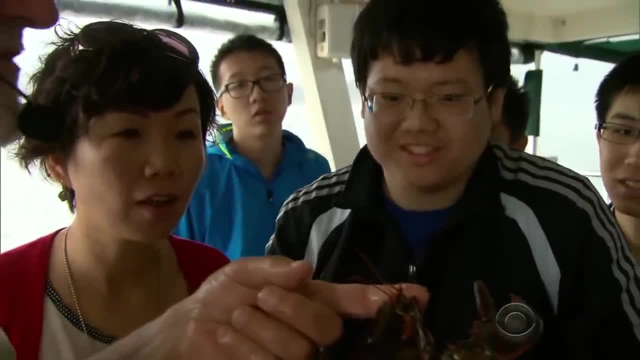 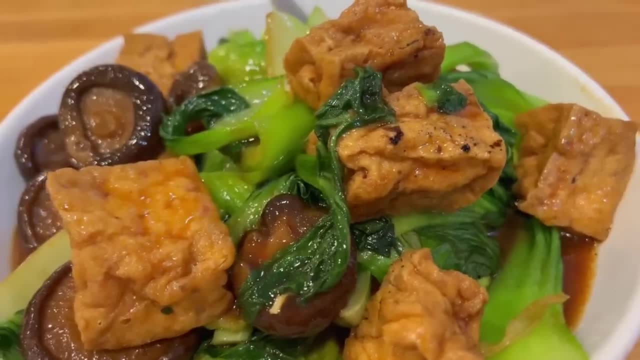 crafts, clothing and more. Unlike some states on this list, the Chinese immigrants in Boston come from all parts of the country, which means the Chinese cuisine is more varied than your typical wonton soup found at many Chinese restaurants that cater to Americans. 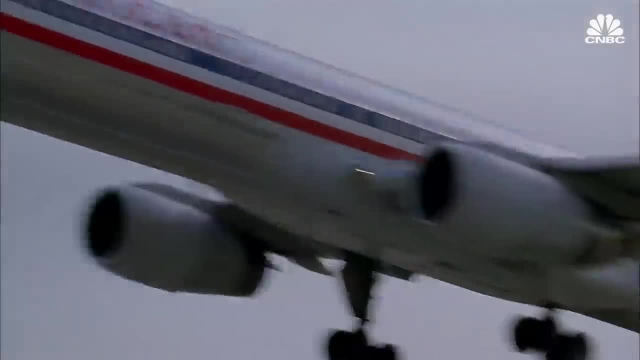 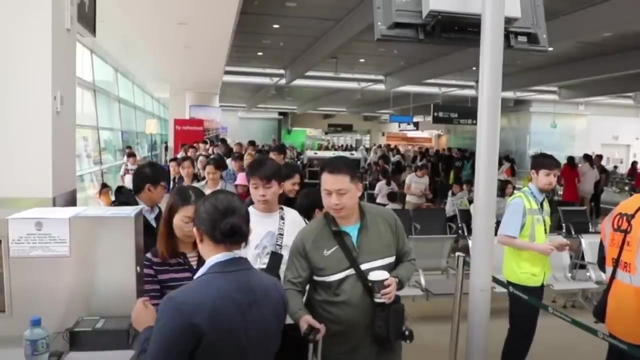 This increase in Chinese immigrants can be seen in the capital, which is a major part of Hong Kong's economy. Hainan Airlines began non-stop service between Beijing and Boston in 2014,, followed by nonstop service between Shanghai and Boston a year later. 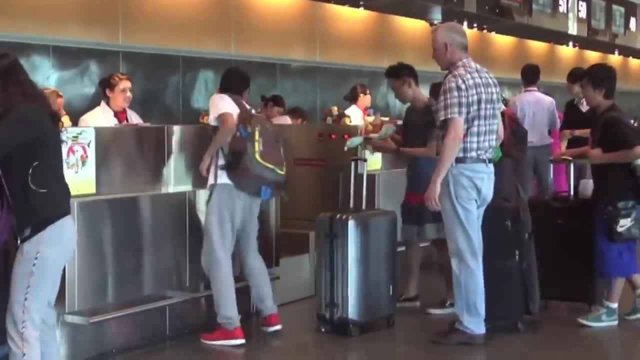 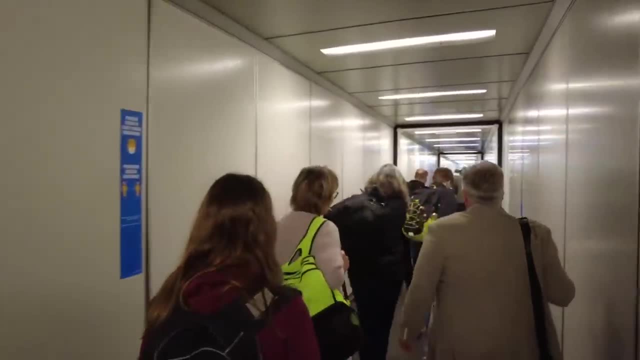 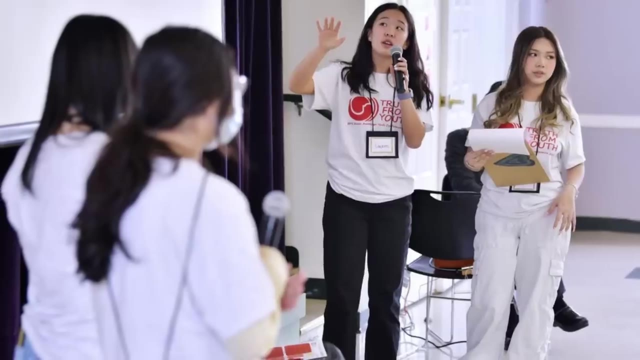 Cathay Pacific Airways also began non-stop service between Hong Kong and Boston in 2015.. These non-stop flight services between China and Boston were not only to cater to the immigrants, but demonstrate the fact that Chinese are the top nationality visiting Boston from outside North America, with nearly 1 in 4 Chinese-American immigrants from the States. 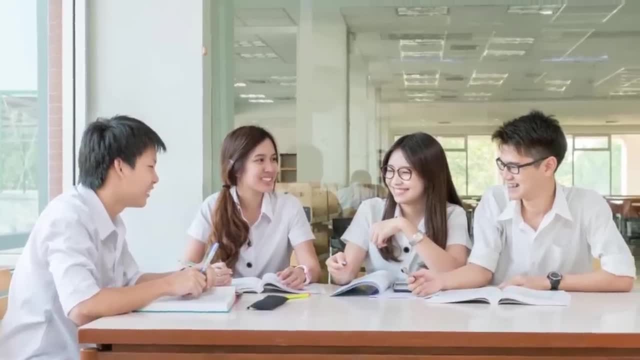 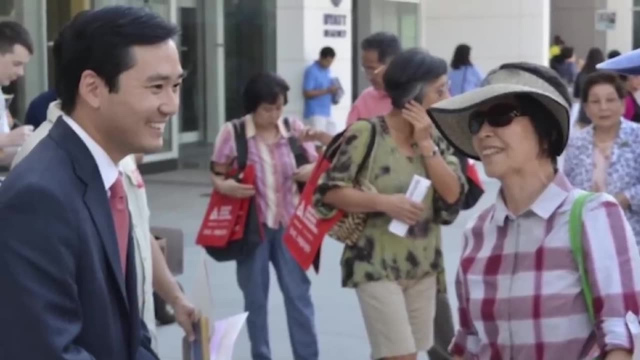 24 Chinese visitors coming to Boston for education. Virginia is for lovers, but it's also for Asian Americans, making it number 8, with 7.9% of its population being Asian. Like Maryland, this is largely tied to its proximity to DC. 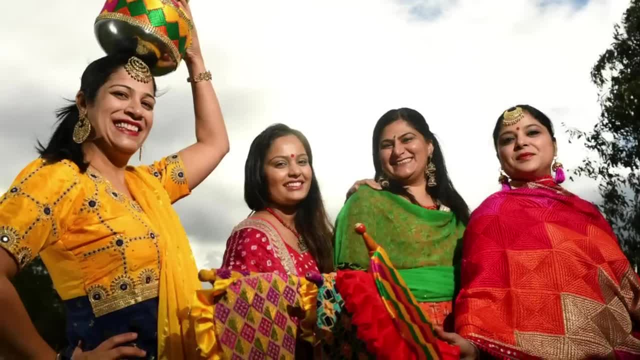 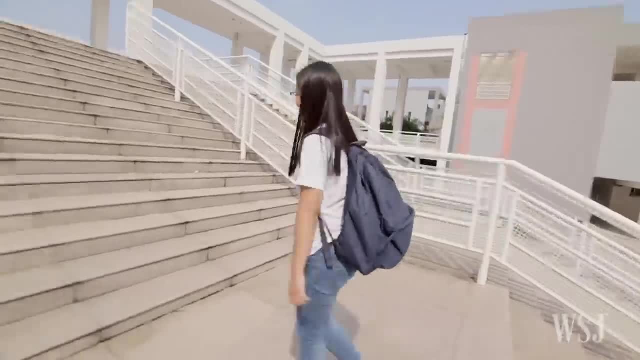 Virginia has a wealth of diversity within its Asian community, with the largest number being from India, followed by South Korea, China, the Philippines and Vietnam. Only 70% of Virginia's Asian population is foreign-born, with many coming for education. 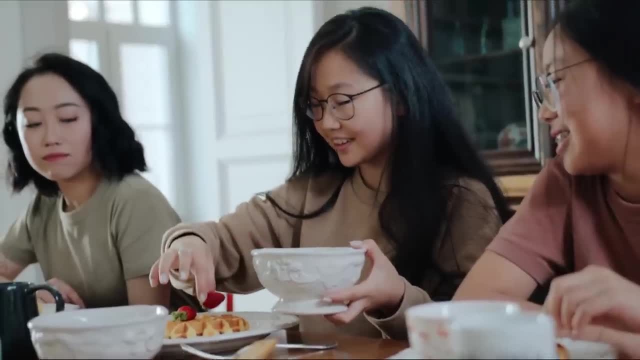 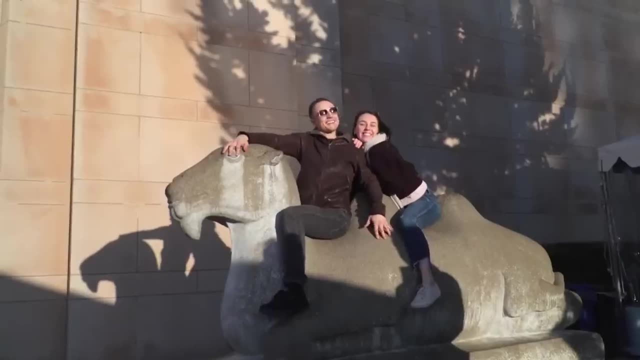 business and to reunite with family. As a whole, Asians have a higher-than-average median home income for Virginia and are more likely to go to college than their Virginia peers. Virginia has many museums dedicated to Asian art and culture, although those in the metro. 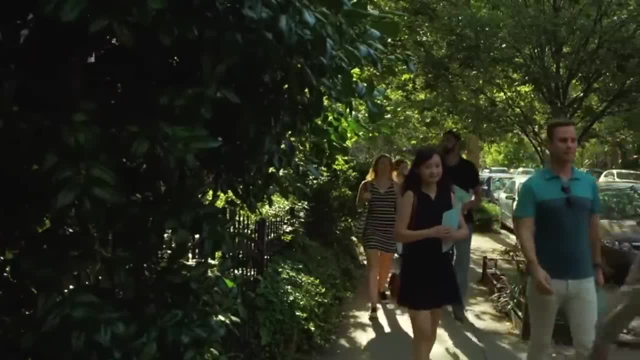 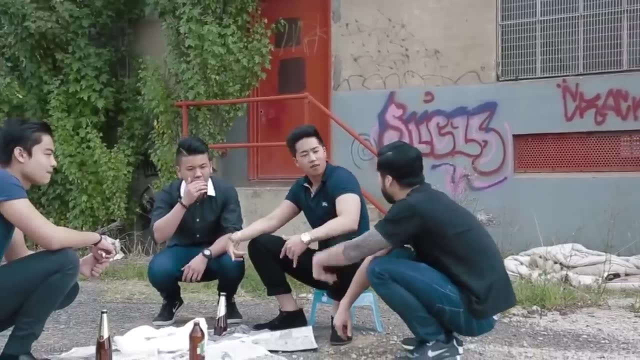 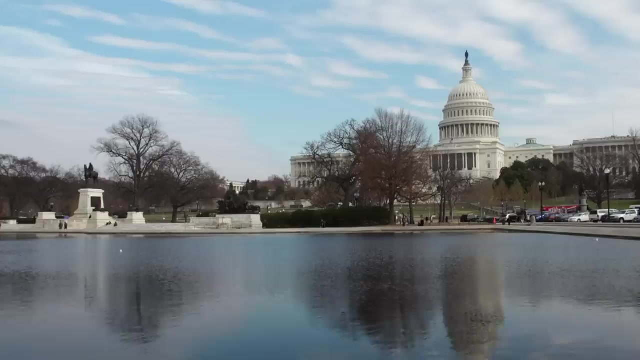 DC area tend to flock to the capital for a wider variety of authentic food and culture, Not counting English, then after Spanish, Chinese and Vietnamese, These are the two most commonly spoken languages in Virginia. The Asian population is disproportionately nestled in the metro DC area, which is to 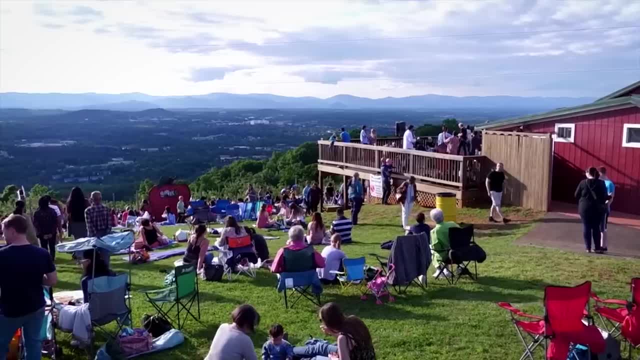 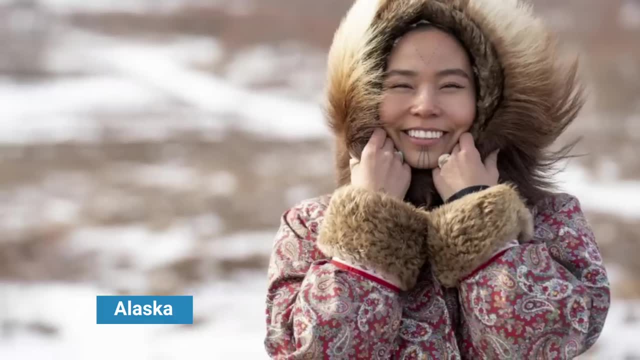 be expected, Much of western Virginia is rural and has far more of a southern culture than a metropolis one. Number 7 is Alaska, with 8.8%. This state should also come as no surprise, given not only its proximity to Asia, but 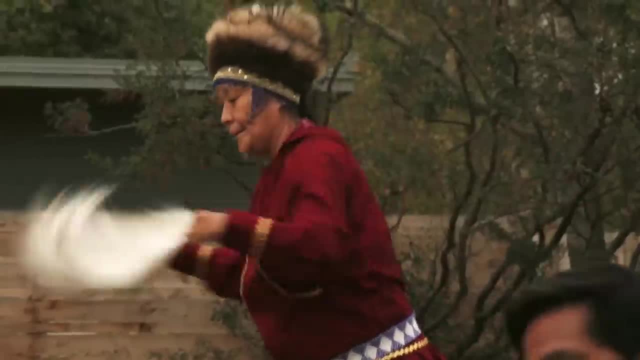 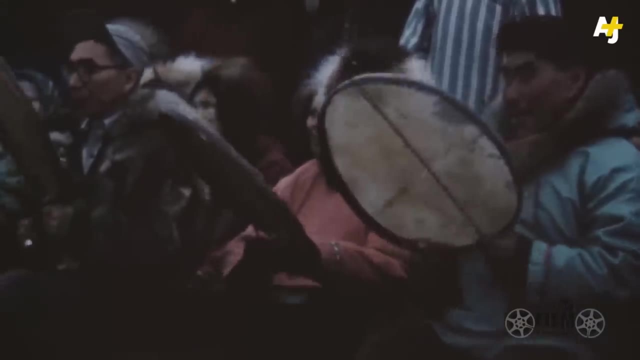 also because its native population can trace its roots to Asia. This is where the US census gets muddy. Alaska, if its native Alaskan and Indian population were counted, should be number three on this list. But, like I said, the US census is complicated. 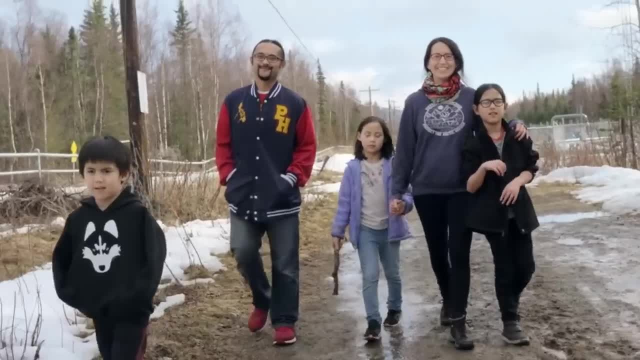 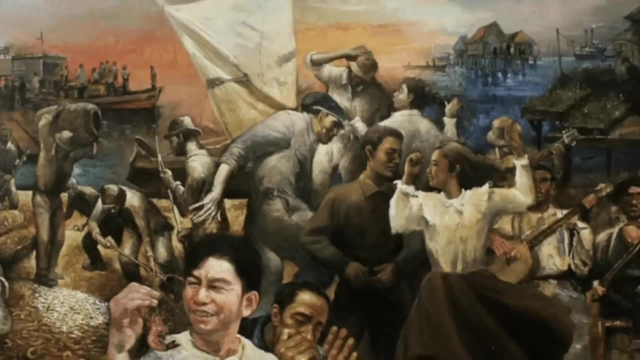 But that's a whole other topic of conversation. Aside from the Alaskan natives, the oldest ethnic group from Asia have been the Filipinos, who have been coming to Alaska since the 1700s. Known then as Manila men, they served as crew members of fur trading vessels. 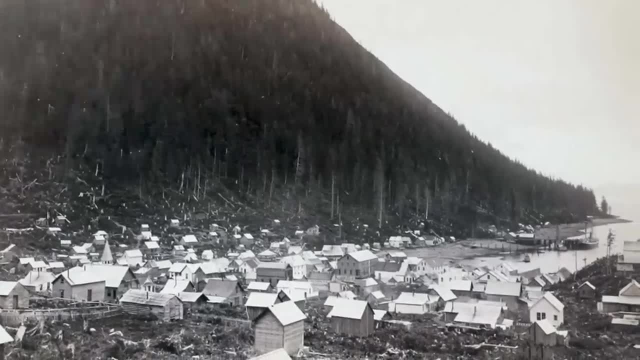 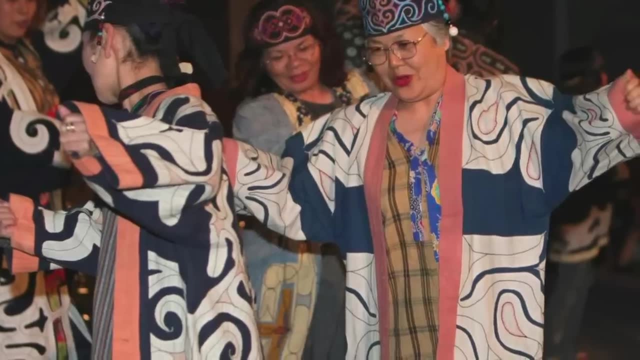 In the early 1900s they largely worked in the gold mines in Juneau. Filipinos still make up the largest Asian subset group in Alaska, followed by Korean, Chinese and Japanese. Anchorage Airport has been a vital refueling hub for cargo flights dating back to the 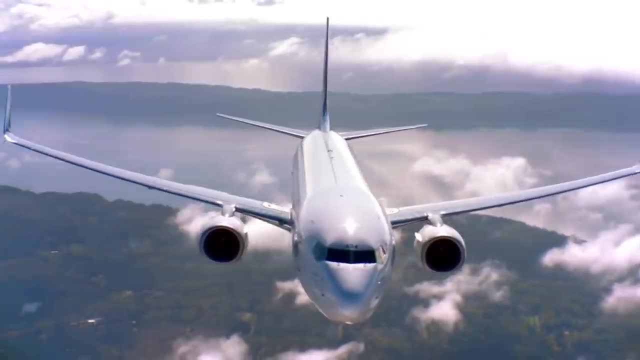 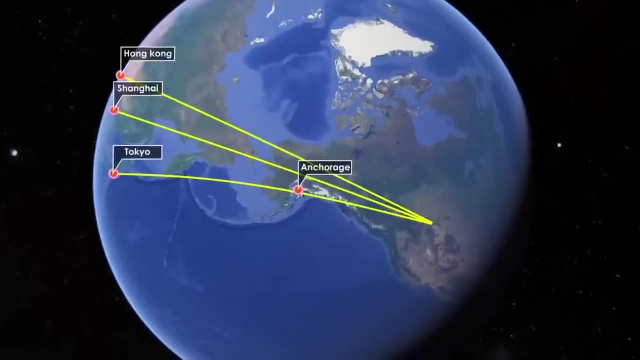 Soviet era, when Soviet airspace was off limits, forcing planes to take longer routes from North America to Asia, All flights coming to and from Asia had to make a pit stop in Anchorage to refuel. The airport has long since been known as the hidden link between North America and Asia. 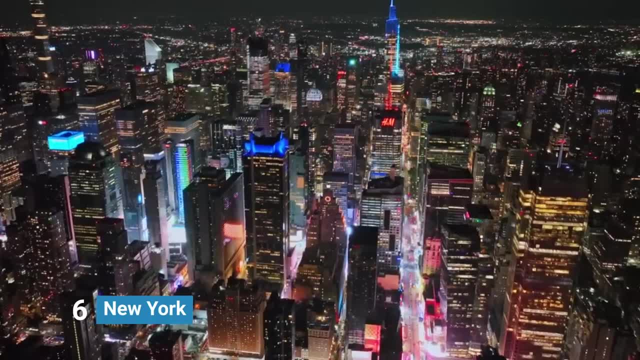 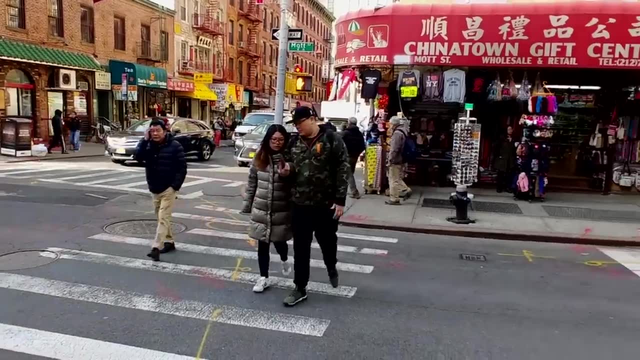 Number 6 is New York, With 9.6%. this should come as no surprise, as New York City is one of the most diverse metropolises in the entire world. Manhattan hosts the world's largest Chinatown. the Empire State Building actually sits in. 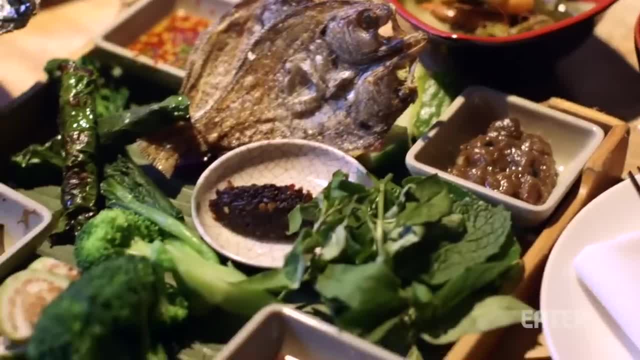 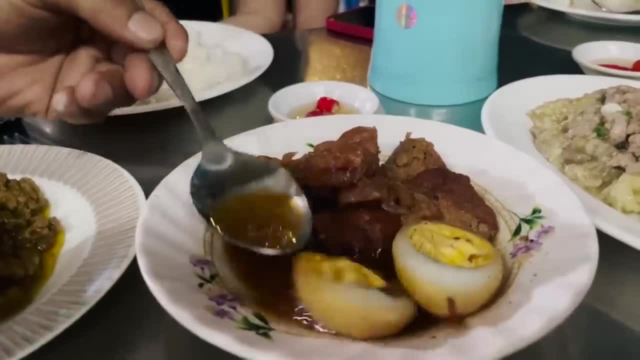 Koreatown, and Laotian food isn't hard to find. Hungry for something from Tibet, Come to New York. Ever wonder what authentic Cambodian food was like? Come to New York. New York City even boasts North Korean cuisine which is different from what we would see. 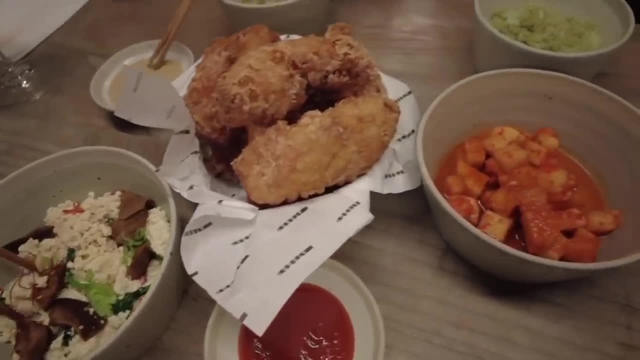 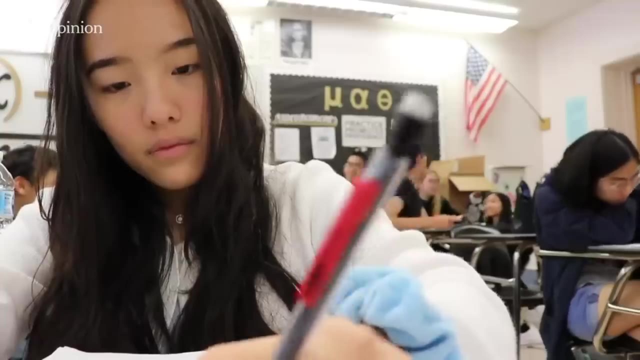 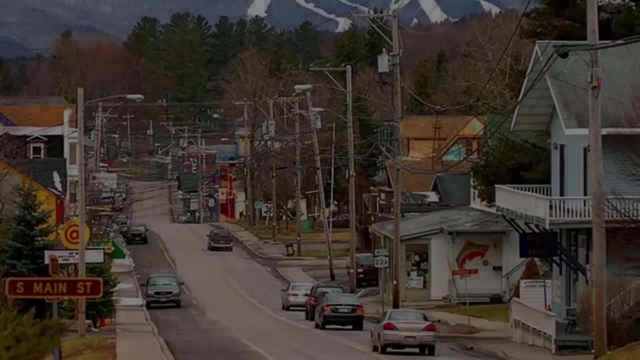 in typical Korean restaurants. There are more than enough museums that feature Asian art and culture, as well as language schools and churches with offerings in just about any Asian language you desire, And it's not just New York City. Upstate New York is rapidly becoming more diverse, with Erie, Albany and Onondaga counties. 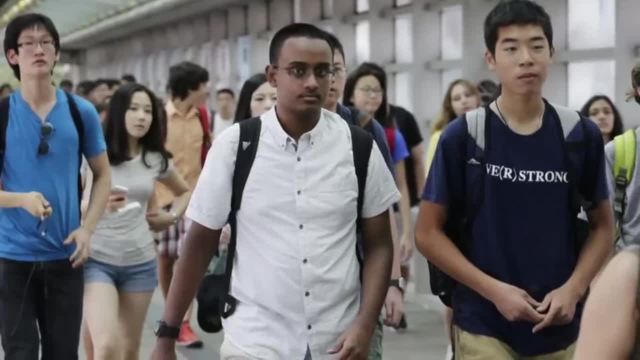 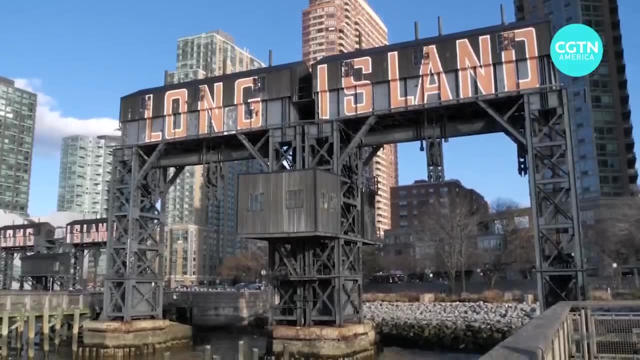 having a large population of Asian Americans and other recent immigrants, Many Asians who want to leave the city for the suburbs are also moving out to Long Island in record numbers. New York has always been a hub for immigration, and those coming from Asia are no exception. 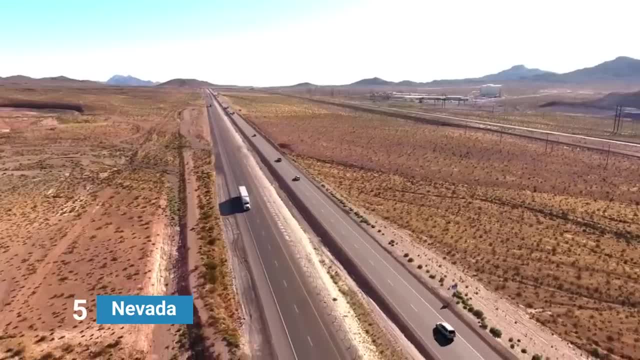 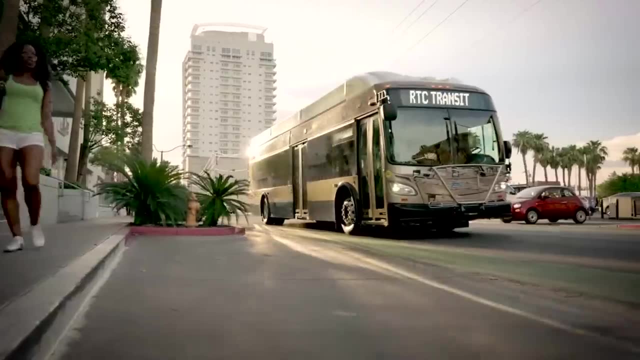 Number 5 is Nevada, with 10%. This one may come as a surprise, as Nevada is largely desert and sparsely populated in most regions beyond Las Vegas. The largest Asian ethnic group in Clark County, home of Las Vegas, is Filipino, followed by 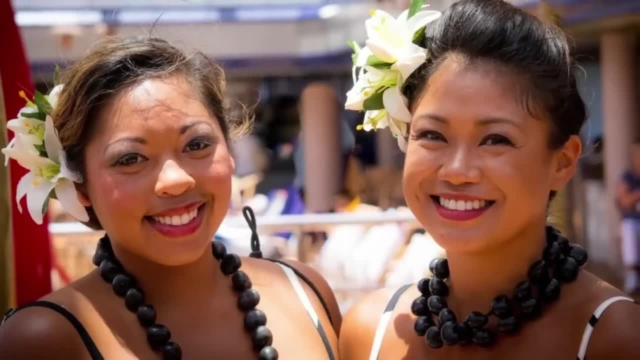 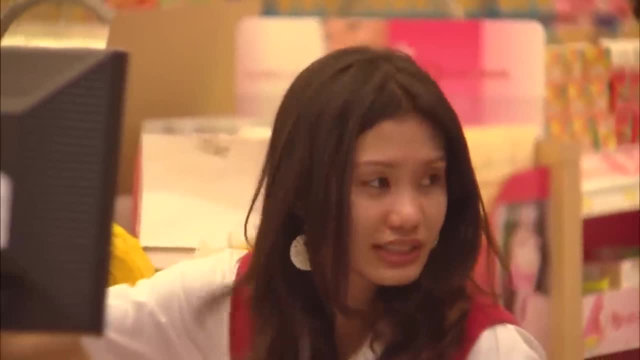 Chinese and then Hawaiian-slash-Pacific Islanders. Nevada is one of only five states where Asians have reached 10% of the population. In both the United States and the United States, Nevada is the largest Asian ethnic group in the world. Both the US and Nevada Asians are the fastest-growing demographic group. 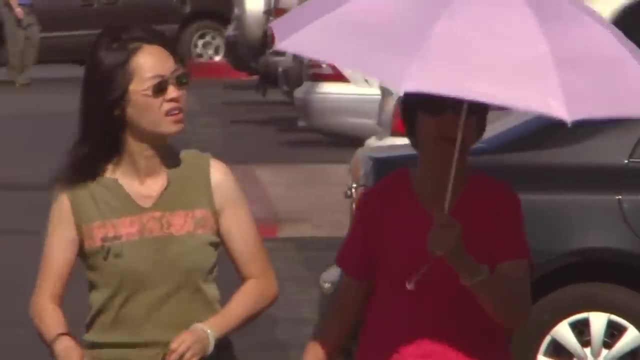 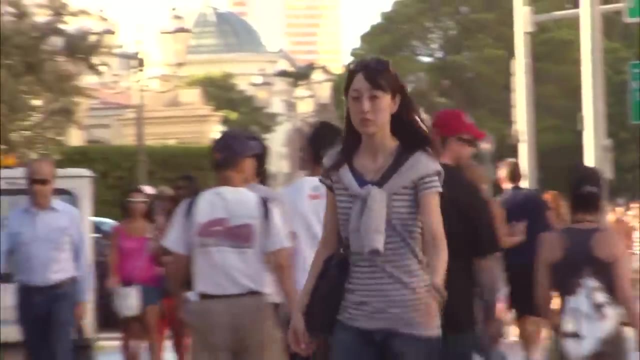 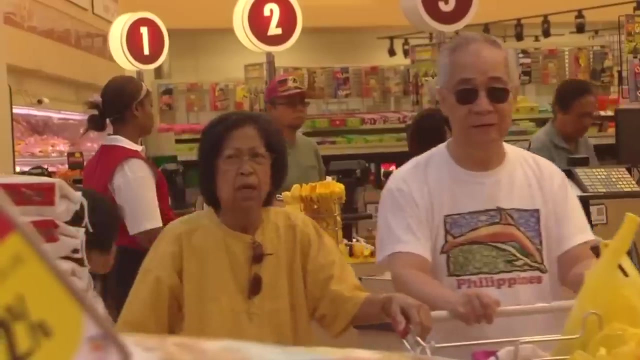 Between 2000 and 2020, the Asian population doubled nationwide, Despite their achievement and high educational attainment. this stereotype of Asians being the model minority has masked the disparities within the Asian community, once again reminding us that Asia is a continent, not a monolithic ethnic group. 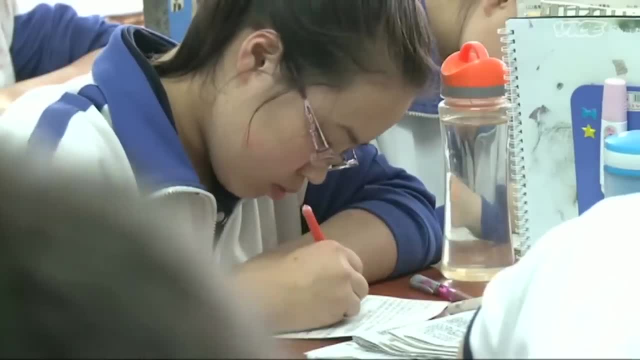 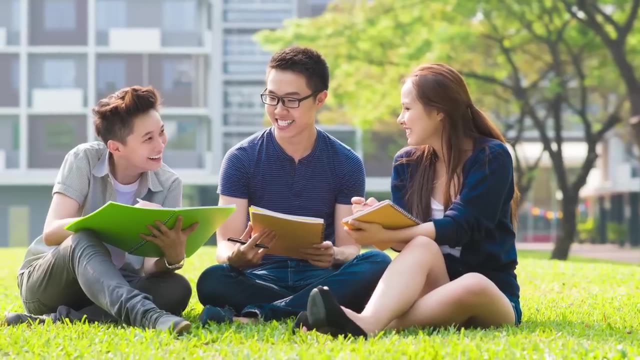 Asian and Pacific Islanders in Nevada have far exceeded their peers when it comes to education. They have a 95% graduation rate. They also accounted for 14% of the gifted and talented programs. However, as the pandemic showed us, Asian Americans are not immune to hate and racism. 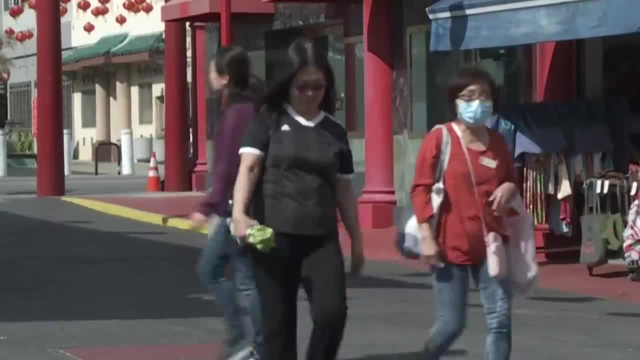 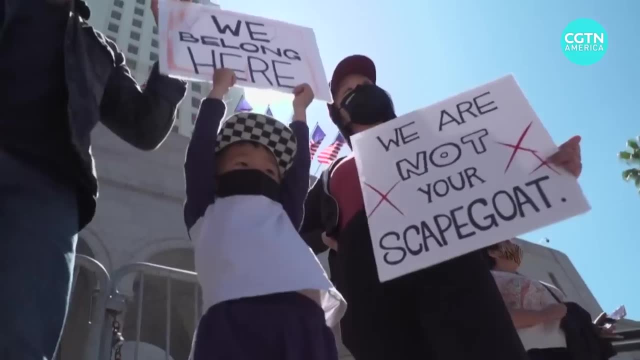 despite their achievements. The Asian, American and Pacific Islander community in Nevada have been fighting hard since the pandemic to bring awareness to the disparities and need for resources within their community. Despite their higher-than-average incomes, they also disproportionately represent those without health care and those who are unhoused in the community. 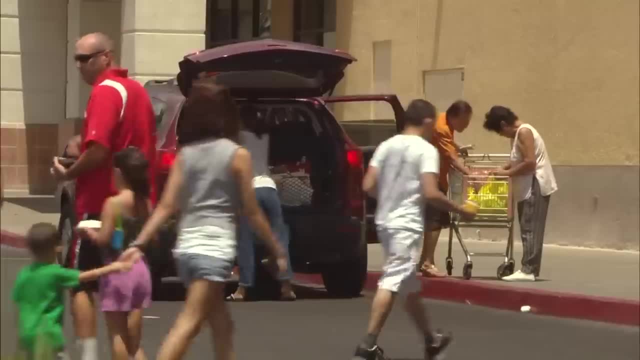 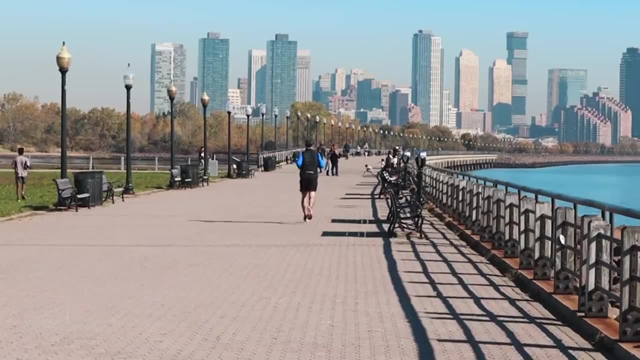 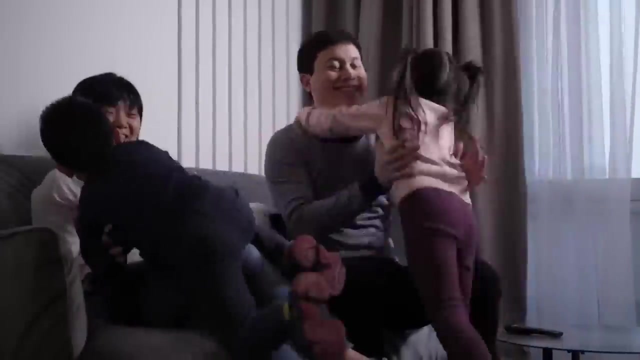 So there is work to be done. 4. New Jersey, with 10.2%. This is no surprise given its proximity to New York City, as northern New Jersey is part of a greater metro area boasting a wealth of diversity. Like in the rest of the US, Asians are the fastest-growing demographic in the state of 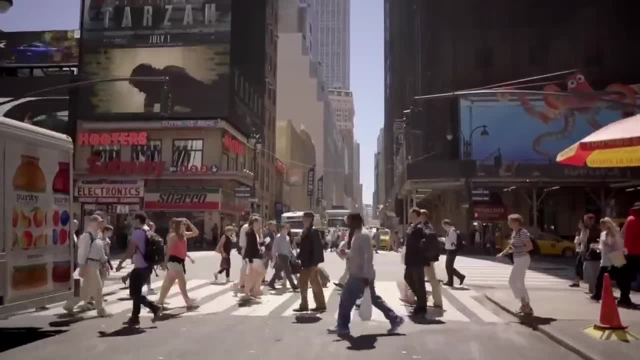 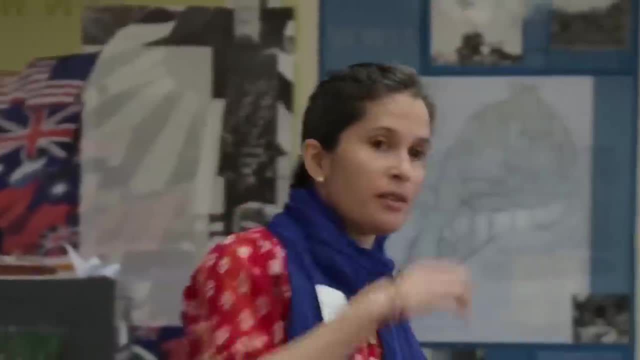 New Jersey. Some of this can be due to many Asians from New York City choosing to move out to the suburbs while still being able to commute to their jobs in the city. In 2022, New Jersey became the second state after Illinois to make Asian American and 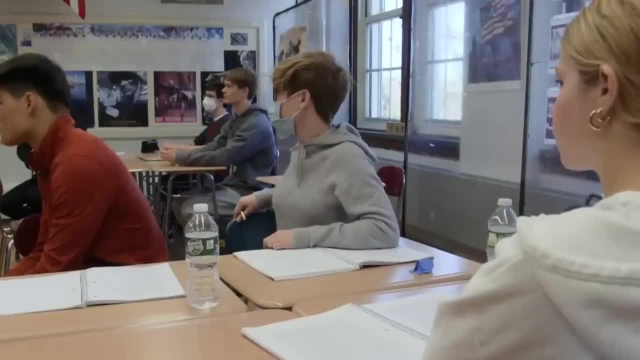 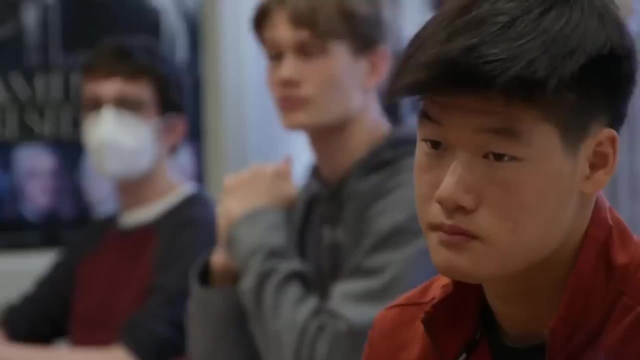 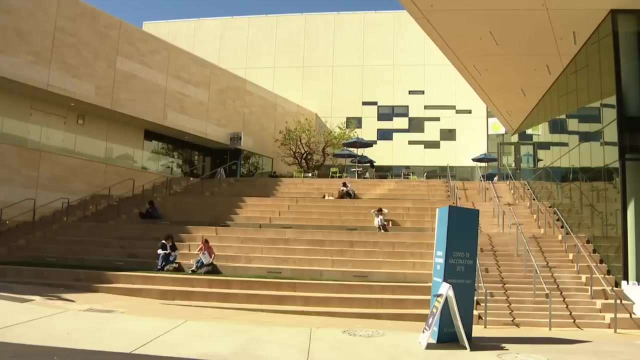 Pacific Island history mandatory in K-12 curricula. This move was due to wanting its schools to better reflect the demographics of the state and, with a population over 10%, it seems only logical that this would be part of American history. Another law will establish a commission for Asian American heritage within the state's 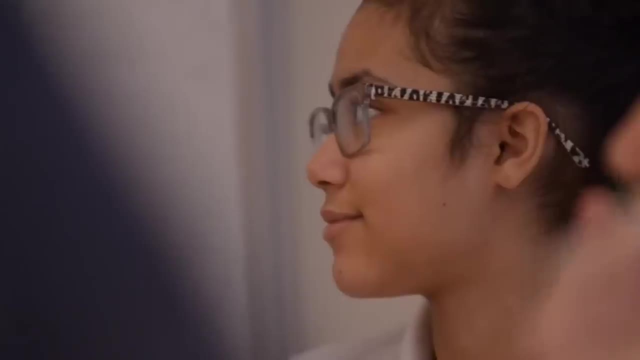 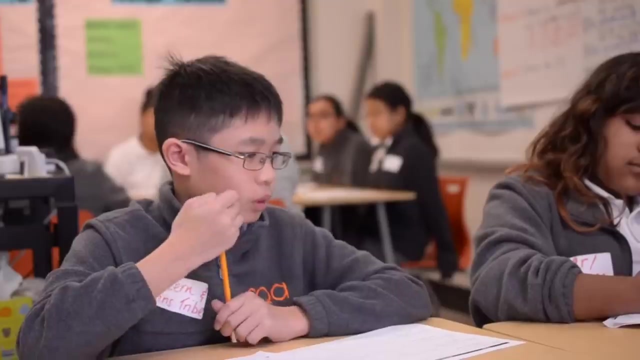 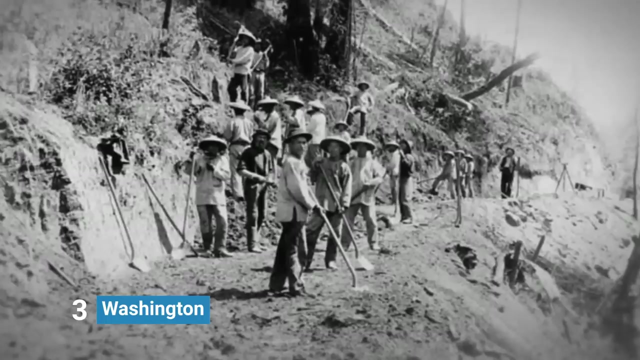 Department of Education, with the expressed purpose of partnering with local schools as they implement this new curriculum. It's important that the history and culture be taught accurately and with proper sensitivity to those communities. Way to go. New Jersey. 3. Washington with 10.9%. Much of the Pacific Northwest has a rich history. of Asian immigration from Alaska down to Vancouver to Seattle, all the way to San Diego. The largest Asian ethnic group in Washington's state is Chinese, followed by Japanese, Korean, Vietnamese, Indian and then Filipino. The Chinese were the first Asian ethnic group to migrate to Washington State back in the 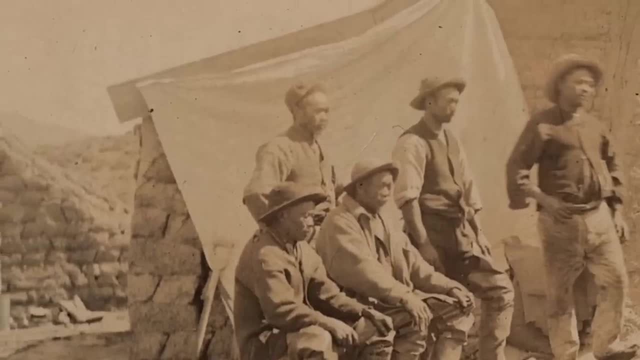 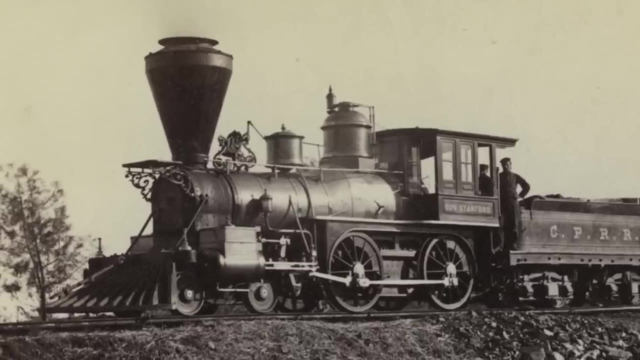 mid-19th century, By the 1860s and 1870s, when gold was struck in the state, many Chinese immigrants came en masse to work in the mines. Sadly, many of these immigrants were also recruited to work on the railroads, where conditions 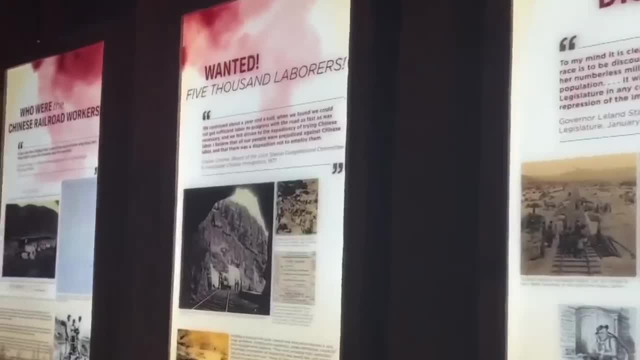 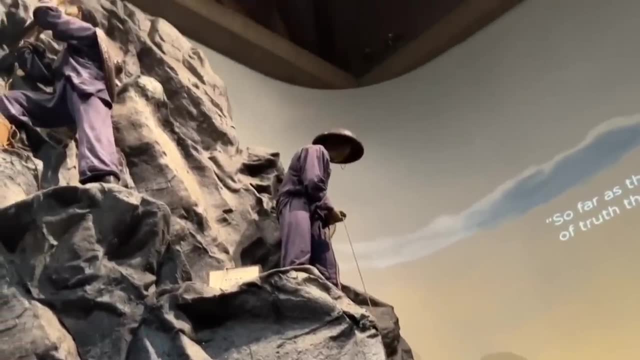 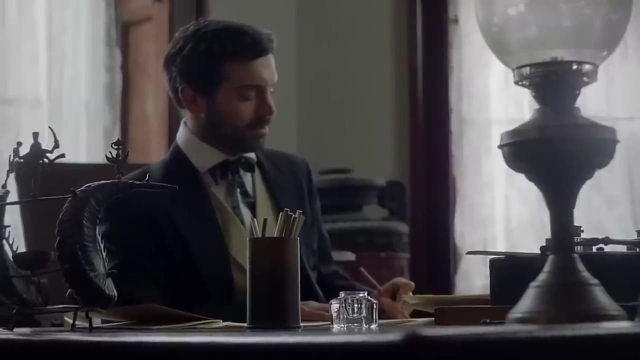 were dangerous and pay was low. The Smithsonian had an exhibit in Washington State, the first of its kind, to honor the forgotten Chinese workers who helped build the Transcontinental Railroad, which opened up the American frontier to the East Coast. This vital piece of infrastructure set in motion the building of a superpower nation. 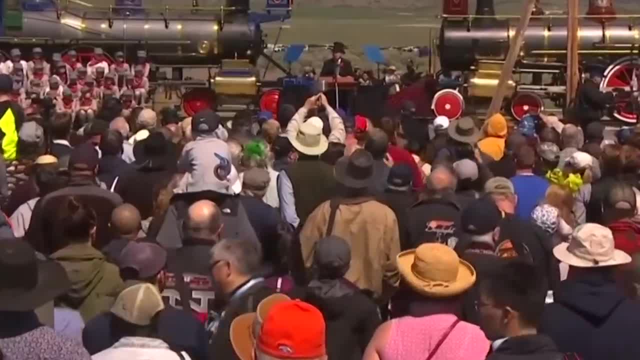 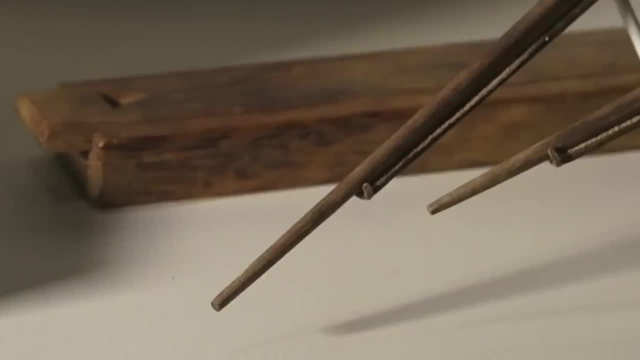 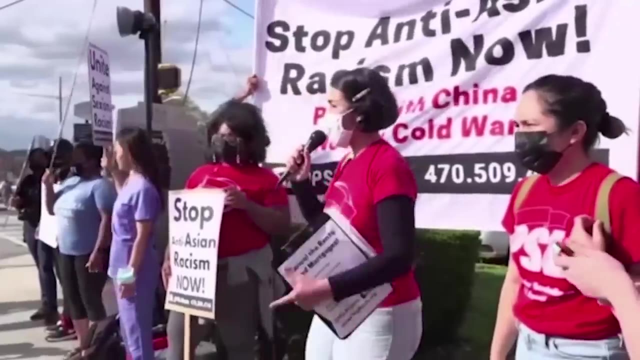 spanning from the Atlantic to the Pacific. 2019 marked the 150-year anniversary of the completion of the railroad, so Washington has made sure to honor those for whose backs the railroad was built upon. Though the Chinese got economic opportunity, they also faced hatred, racism and legal 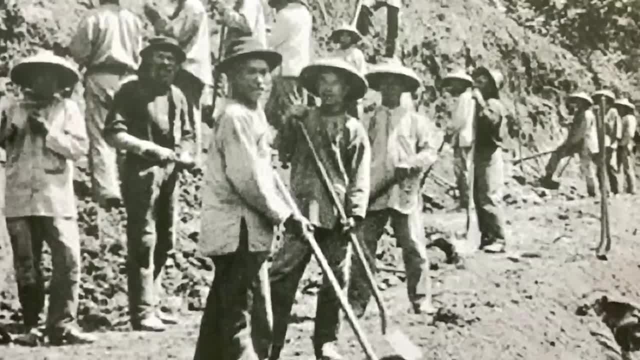 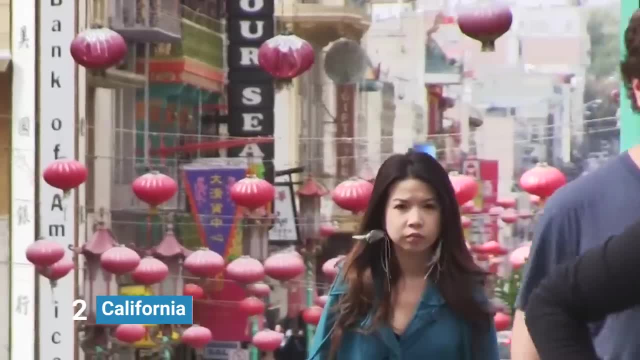 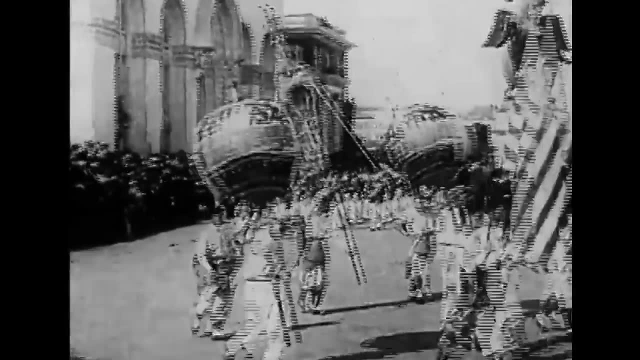 exclusion. The rich history of Asian workers puts Washington State at number three. Number two is California, with 17.3 percent. Though the largest Chinatown is located in New York City, the most famous is undoubtedly in San Francisco. It is also the oldest one, established in 1848. 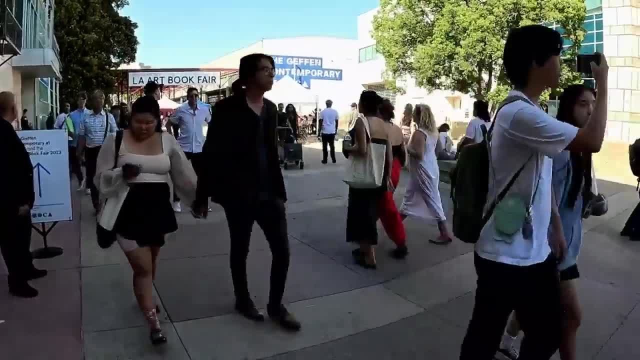 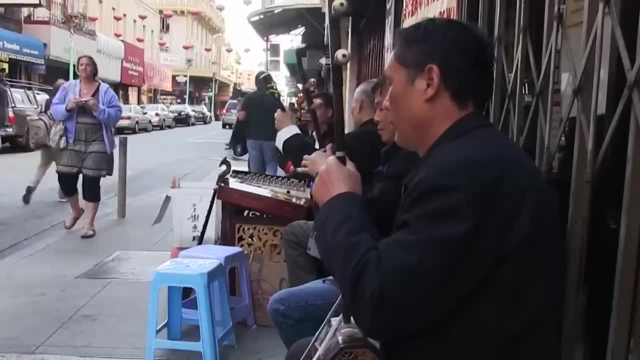 It's hard not to see the influence of Asian culture up and down the California coast when you see landmarks such as Little Tokyo and the Asian Art Museum. This is also prevalent in its food and language. California's Asian population has grown 25-percent. 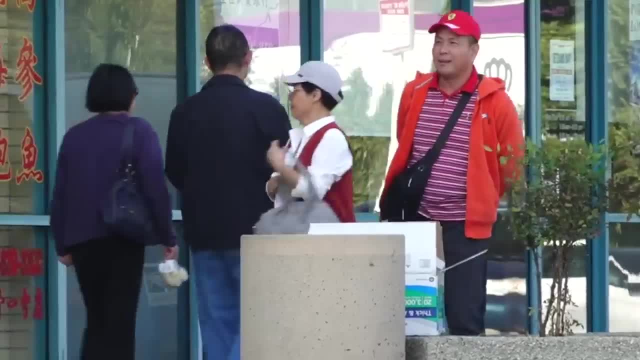 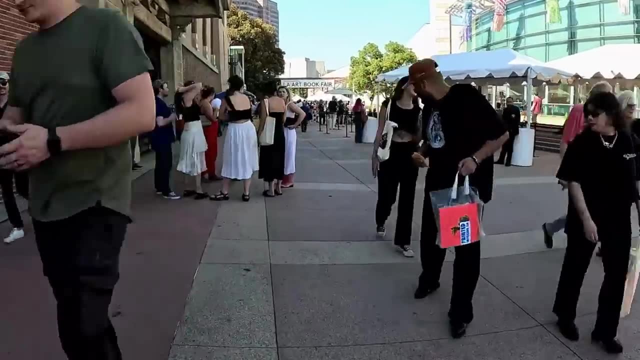 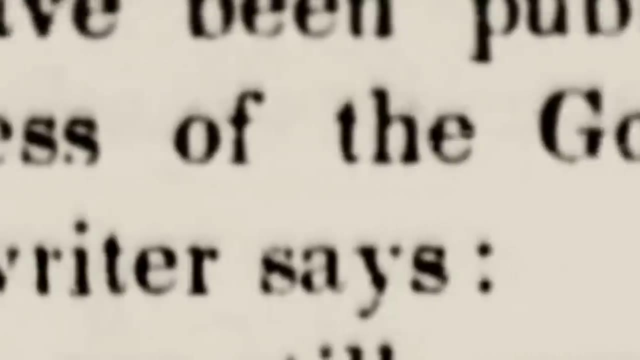 The population of California has grown 25-percent. This has enriched both the cultural and economic landscape of the state. The dominant groups are Filipino, Chinese, Vietnamese, Indian, Korean, Japanese, Taiwanese and Cambodian. This diverse mix of ethnic groups has been a rich part of California's history since. 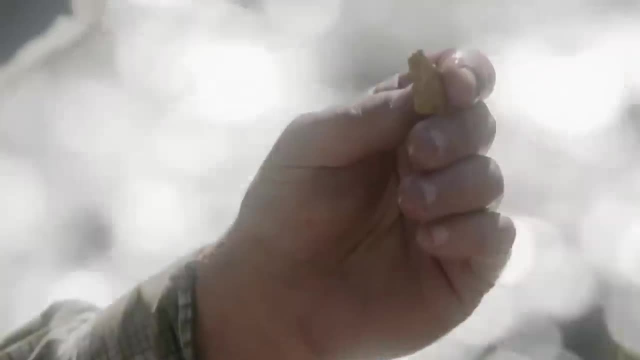 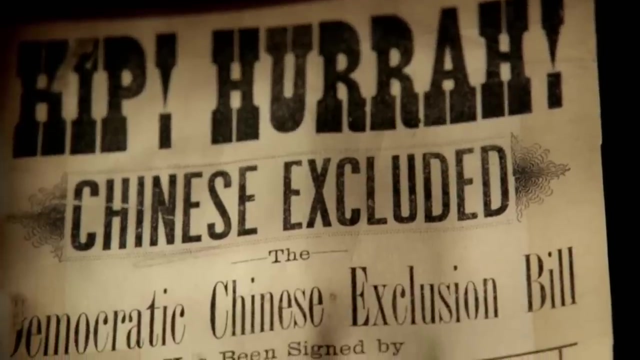 the mid-1800s, when the first Asian immigrants arrived in the Golden State. These newly established communities faced a lot of adversity throughout the decades, from the Chinese Exclusion Act of 1882, the internment of Japanese immigrants, to the Chinese Exclusion Act of 1888.. There was also the internment of Japanese Americans during World War II, all the way to the inegibility for citizenship imposed on Asian immigrants until the 1960s, But that hasn't stopped them from thriving in education and business. Before we get to number one, can you guess the state with the fewest Asian Americans? 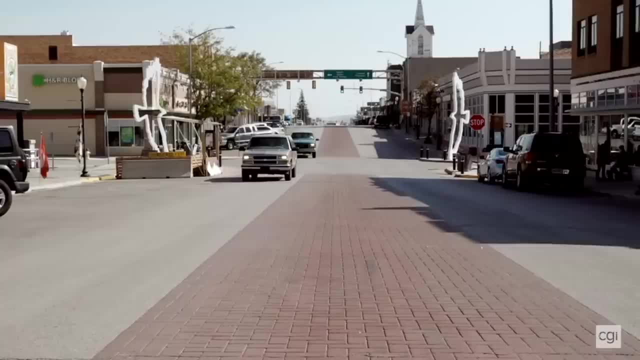 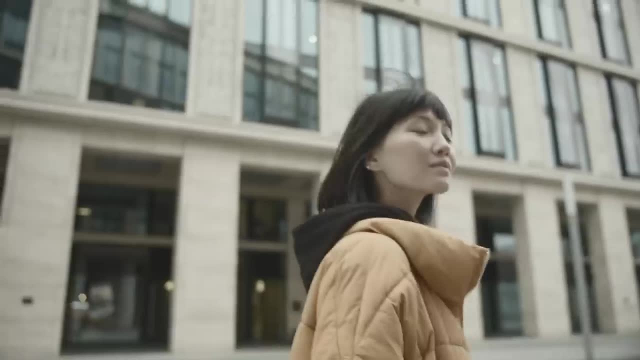 It's also the state with the fewest people period. That honor goes to Wyoming. There are only 4,633 Asian Americans living in Wyoming, making up less than 1-percent of the population. Now let's take a look at the state with the most Asian Americans in the nation. 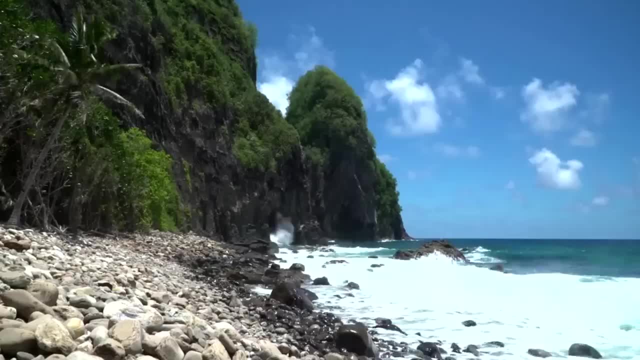 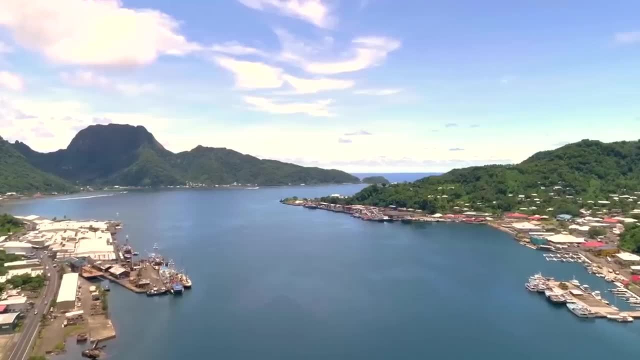 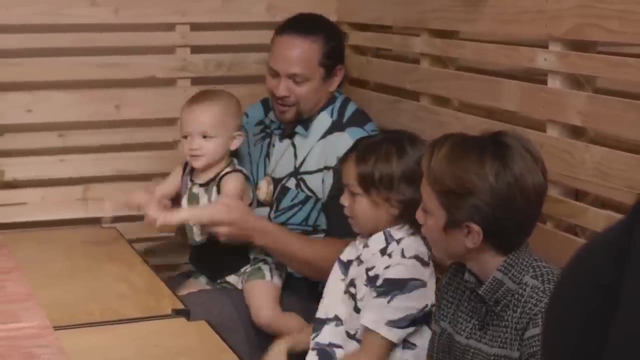 To be fair, if we include US territories, then Guam and American Samoa win by a landslide, which makes sense given that they are in the South Pacific. Speaking of the South Pacific, number one is Hawaii, with 56 percent. This should come as no surprise, given its proximity to Asia, and not to mention that 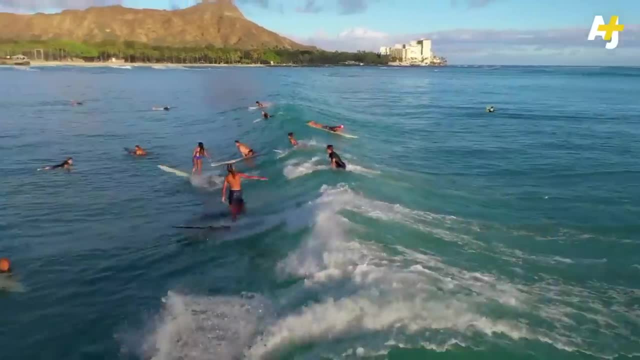 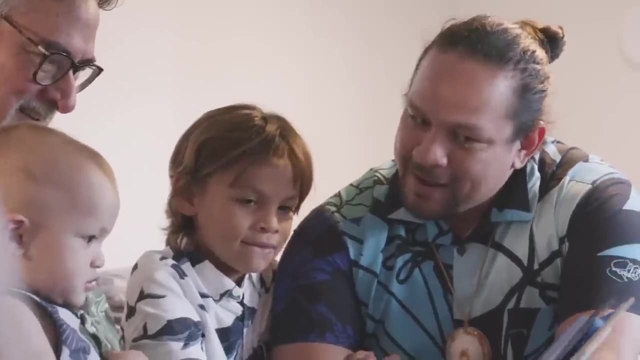 Hawaiian is. in the description from the US Census, Hawaii is a majority-minority state. This means that the majority of Asian Americans live in the United States. while the majority of Asian Americans live in the United States, Most people, while being a national majority, are a minority in Hawaii, with Asian Americans. 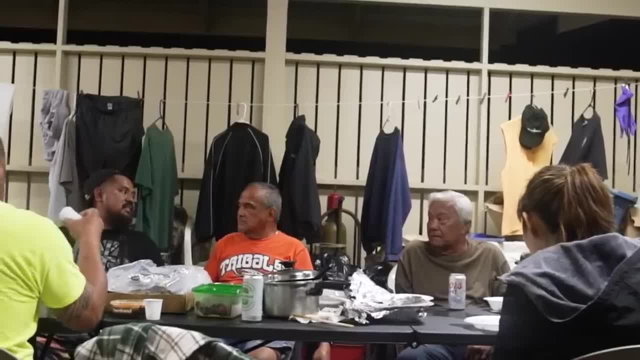 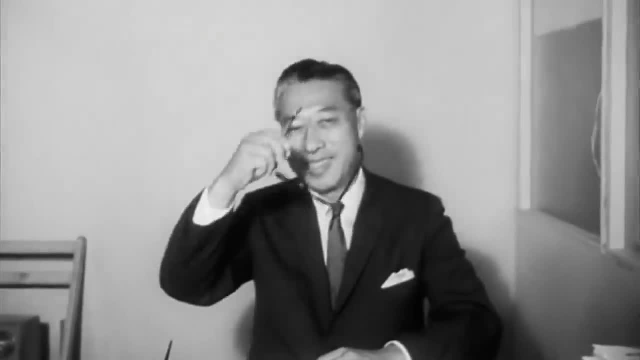 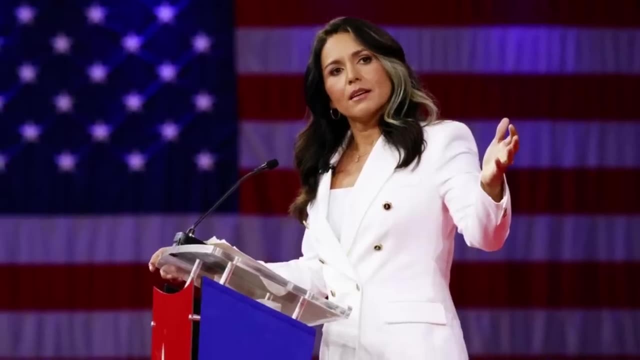 dominating paradise. Asian and Native culture are evident throughout the islands, from its food to even surfing. The first senator of Chinese descent represented Hawaii in 1959, followed by Daniel Inouye in 1963, who was of Japanese descent. The most famous Hawaiian representative of modern times is Tulsi Gabbard, who made history. 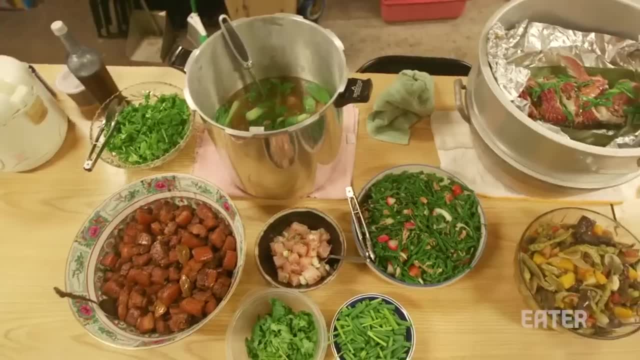 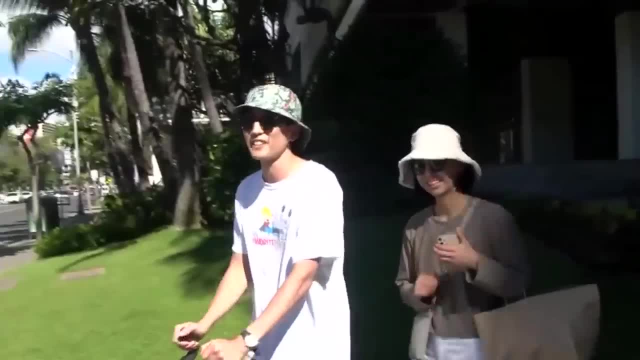 Some of the best food that is native to Hawaii are the local foods. Historic history tells us that at the beginning of COVID 19, Hawaii began to be a certificated, almost organic, salt. current Japanese influence can be seen in many of Hawaii's cuisine as well. 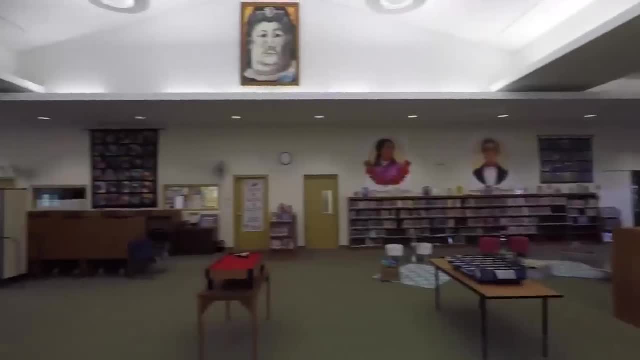 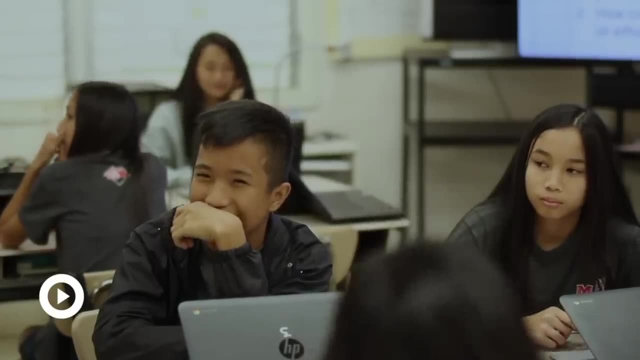 It is not uncommon in Hawaii grade schools to take Japanese, Mandarin or Korean as a foreign language. Students can also learn Hawaiian language and culture in K-12 schools. Did you know that there is a dark side to Hawaii? Click this next video to learn about some of the struggles Hawaii faces.